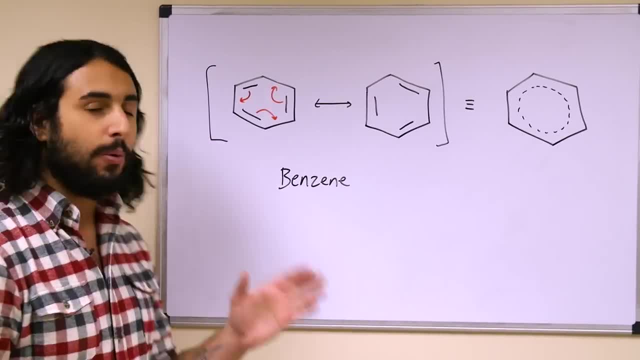 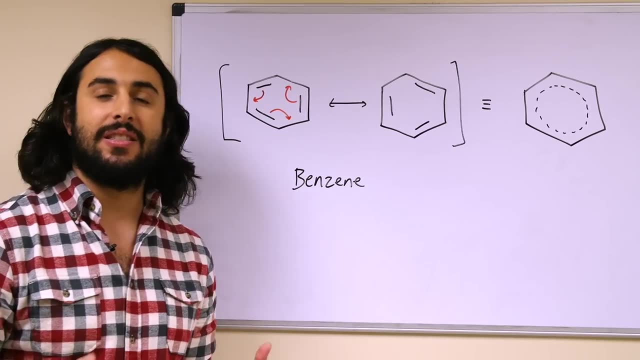 And so let's take a look at what we mean by that. So, if we remember from what we were discussing about resonance, we have this molecule here. we have three pi bonds and we notice that they are conjugated, meaning we have this alternating double bond single bond system. 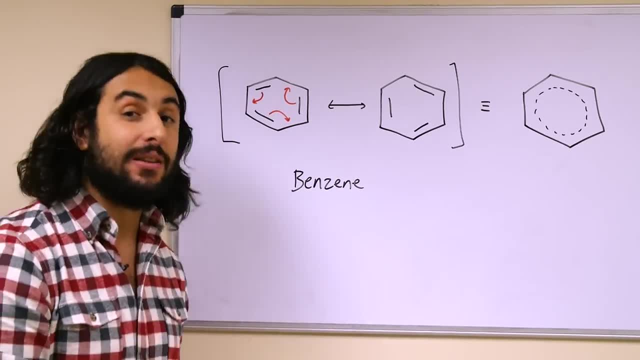 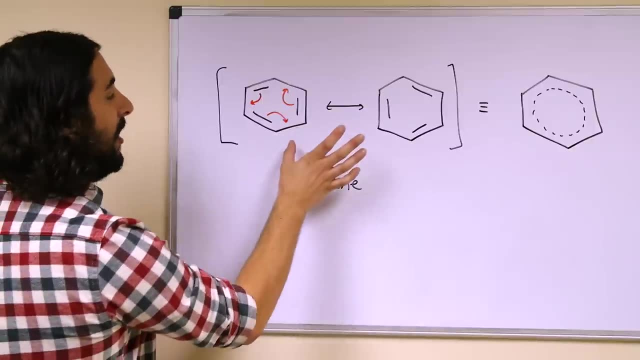 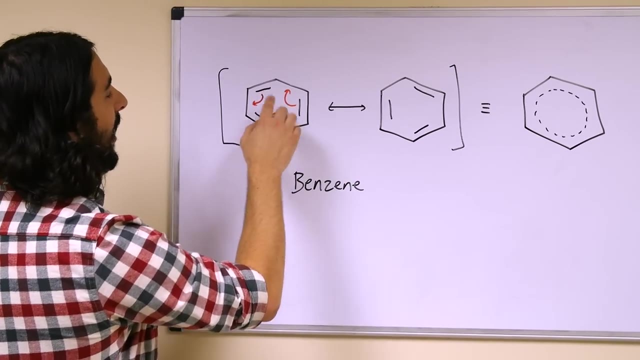 and so these are now fully delocalized. They're not just delocalized about a portion of the molecule, they are actually delocalized around the entire molecule. So we have these two different resonance structures for benzene, and we can see that, given that in each of the two resonance structures, 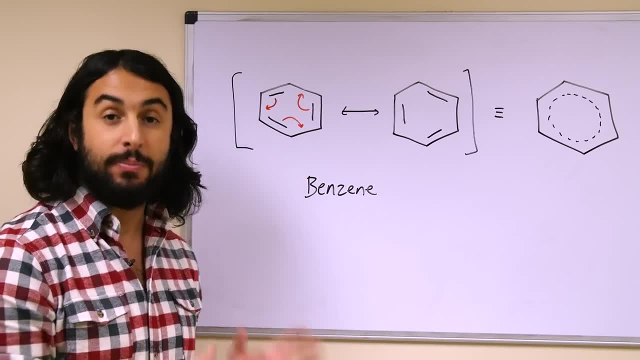 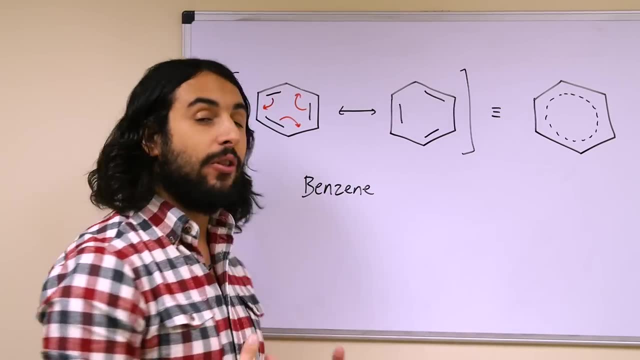 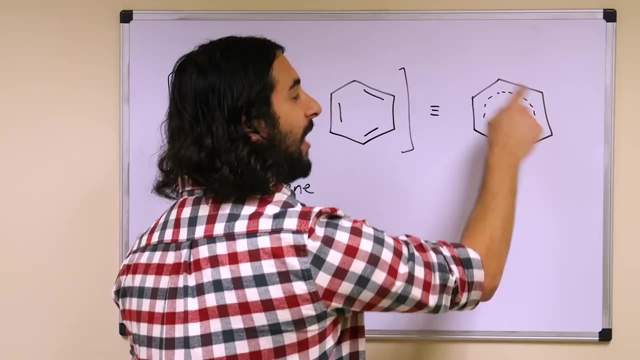 there is a double bond at every single possible position between them, And so that means that recalling the fact that these actually do not exist, but is actually the composite resonance structure that is real. So benzene really looks like this, where we have partial pi electron density. all about the ring. 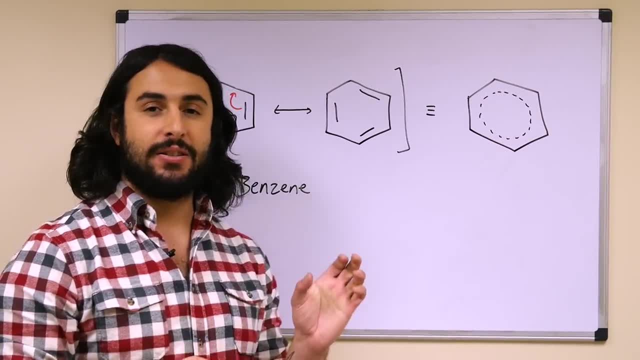 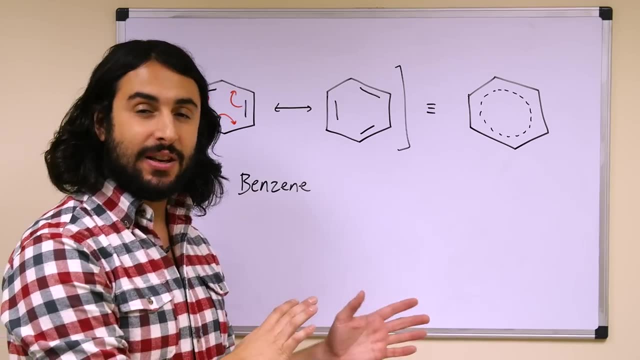 So that's what we mean when we talk about a ring system that is fully conjugated and unsaturated, So that is a prerequisite for aromaticity. It's not only benzene that is aromatic, but it's the most common example, And so what we want to do now is take a look at some rules to help us determine. 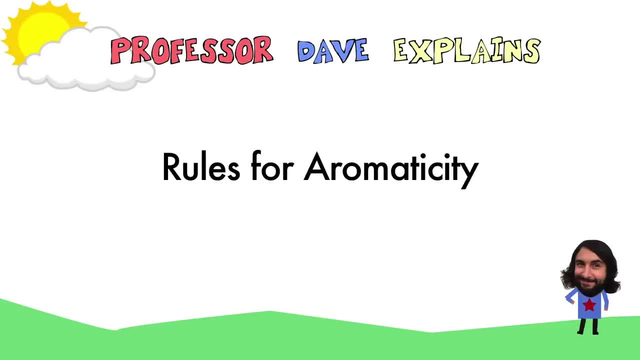 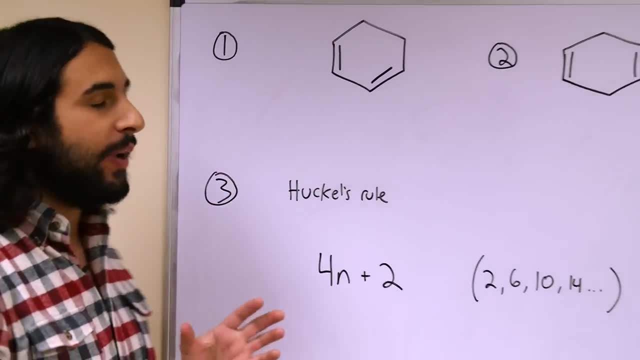 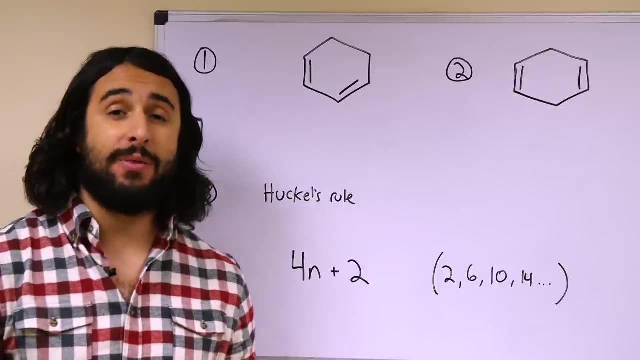 whether a molecule is or is not aromatic. So let's take a look at the rules for aromaticity. Number one: the ring system in question must be fully planar. So, looking at something like this, there's a portion here that is sp3 hybridized. 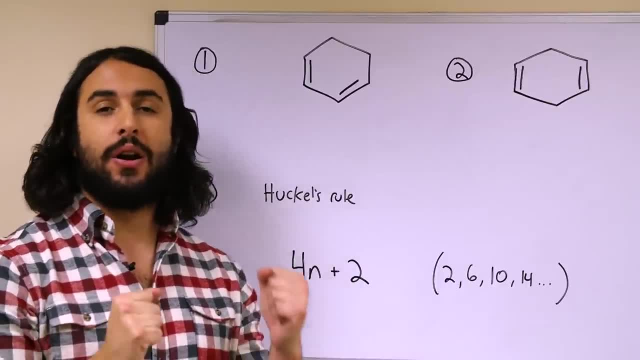 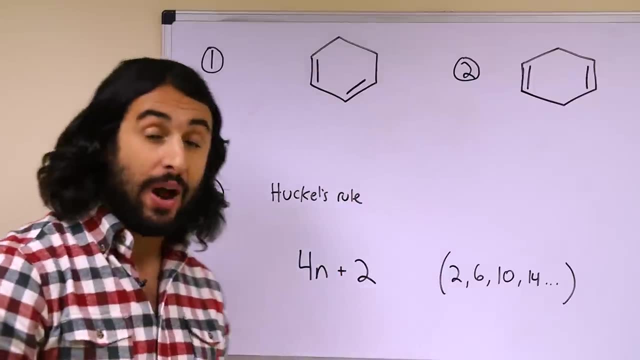 and therefore has tetrahedral geometry. So there are groups that are projecting in and out of the board, So that is not fully planar. We must remember that only the carbons that are sp2 hybridized will have trigonal planar geometry and therefore can be. 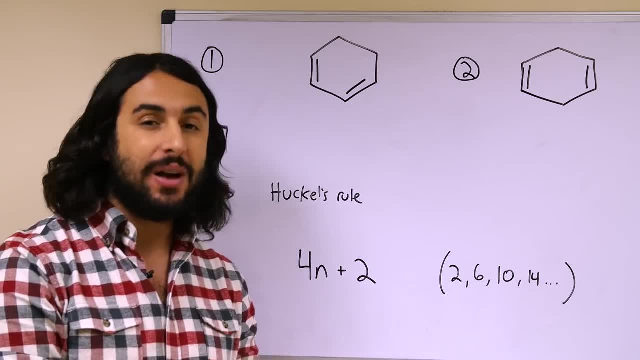 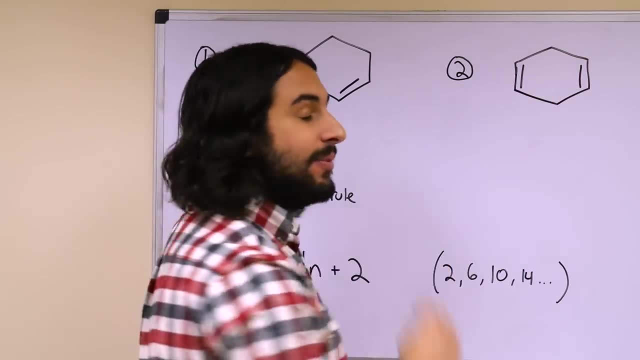 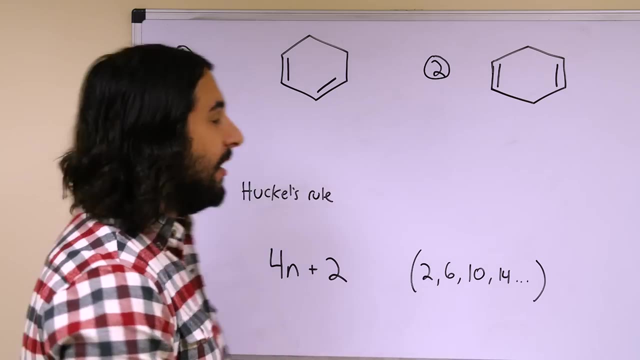 the molecule could be considered planar, So the entire molecule must be planar. Number two, the system must be fully conjugated. So while, in addition to the fact that these are sp3- hybridized carbons- also these pi bonds are not situated in a way that makes the system conjugated. 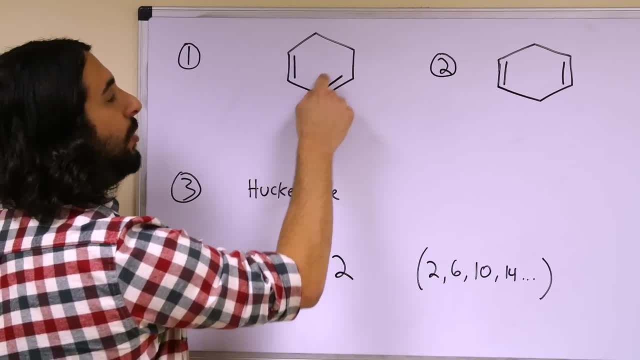 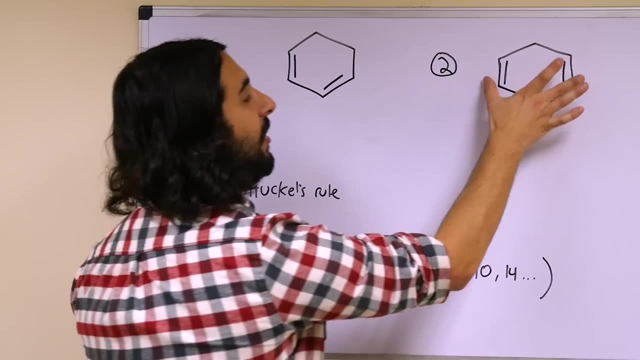 Remember that at least here there is some delocalization of these pi electrons, because they are arranged in the appropriate fashion, alternating double bond and single bond. Here these are too far apart for these to be conjugated, So this could not qualify as aromatic. 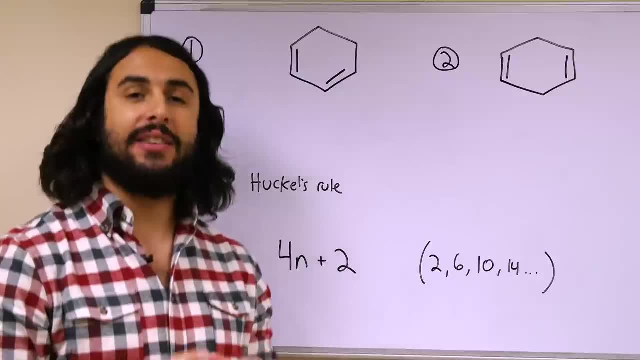 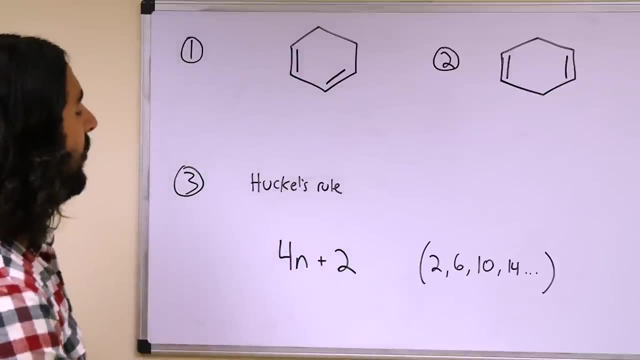 And then the last thing is that the number of pi electrons present that are delocalized must obey Huckel's rule, And Huckel's rule is as follows: We have this term, 4n plus 2, where n could be any integer. 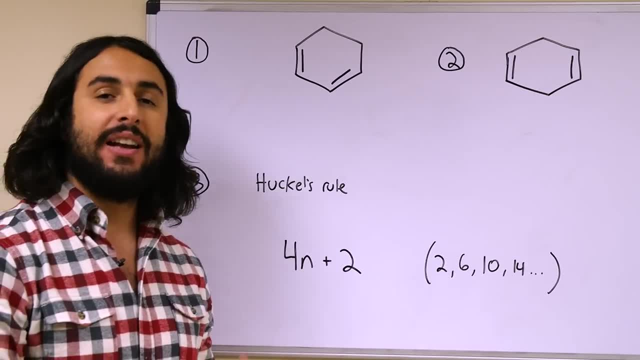 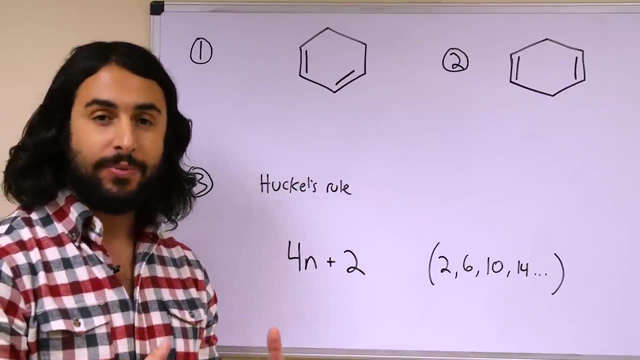 And for whatever integer you put into Huckel's rule, it spits out a value for a number of pi electrons that are delocalized. that will generate an aromatic system. So that sounds more complicated than it is. Let's put in any integer. 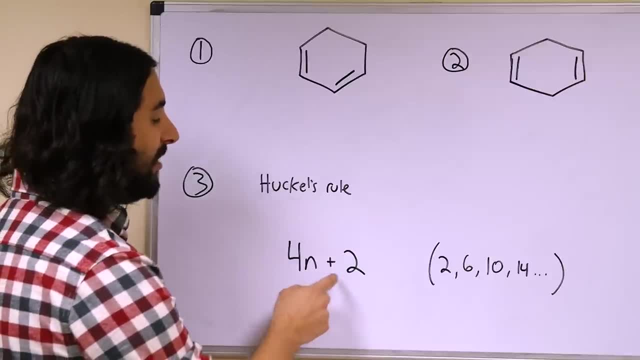 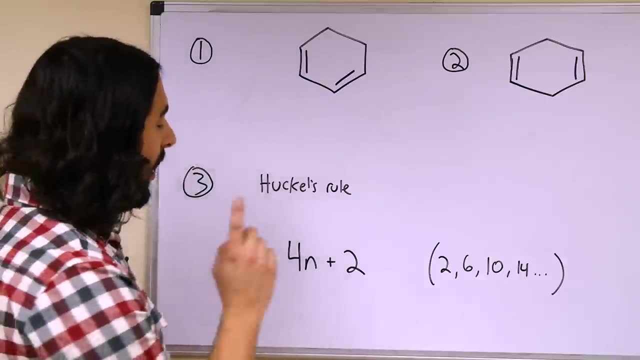 Let's say 0. If n equals 0,, 4 times 0 plus 2 equals 2.. That means that a system with 2 pi electrons could be aromatic. Let's put in the number 1. Then we'll have 4 plus 2, or 6.. That means that 6 is a number of pi electrons in the system that could promote aromaticity. So we end up with this: 2, 6,, 10,, 14. And so forth, And so those are the values that allow for aromaticity. 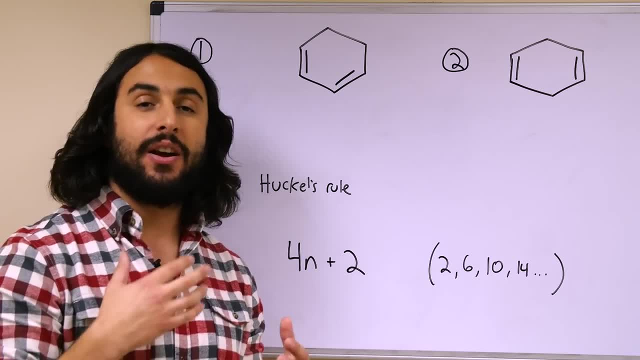 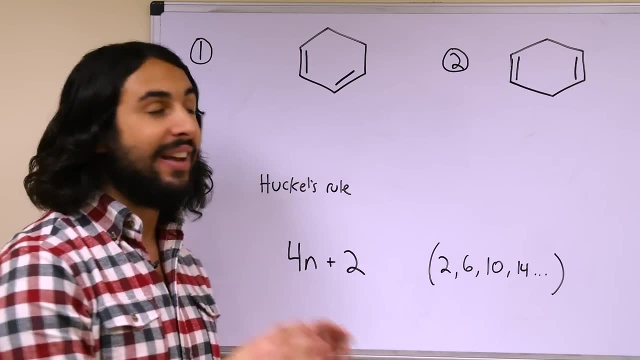 when we're looking at the number of pi electrons that are delocalized within the system, So 4, 8,, 12, etc. Those, even if the molecule is fully planar and fully conjugated, will not be aromatic. 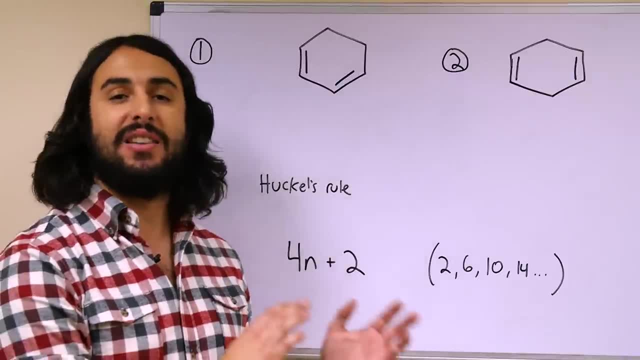 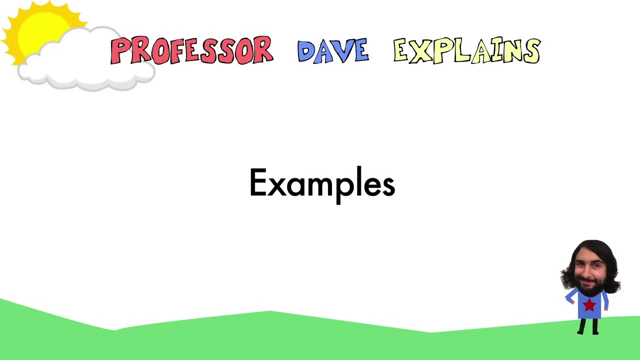 So let's take a look at a couple of examples and apply these rules and see if we can predict which are going to be aromatic and which are going to be anti-aromatic. So let's take a look at some examples. So first of all, we have this 3-membered ring here. 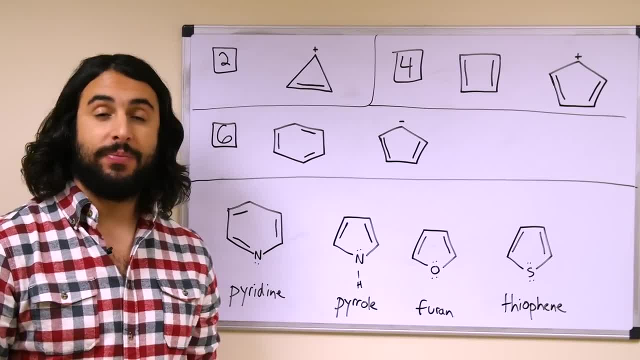 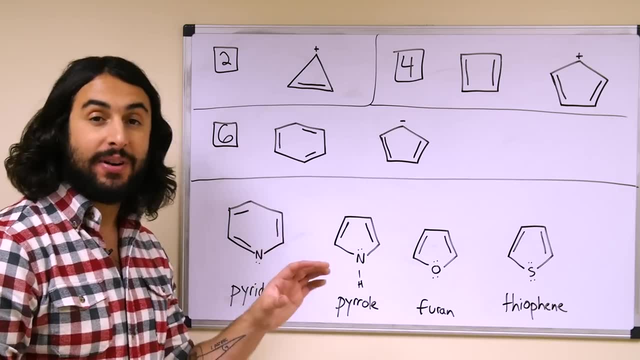 And this is fully planar and it is fully conjugated because we have a carbocation up here. So that makes that sp2 hybridized and planar. And it is fully conjugated because we can move this single pi bond around the molecule. 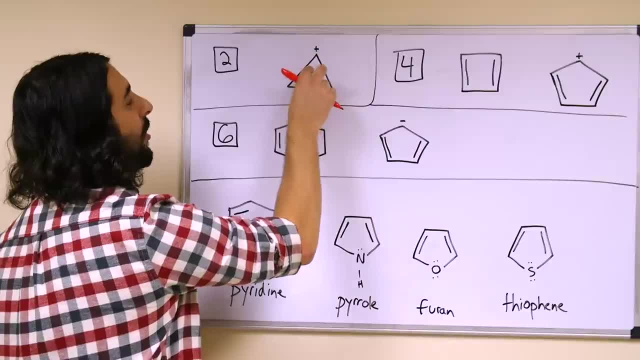 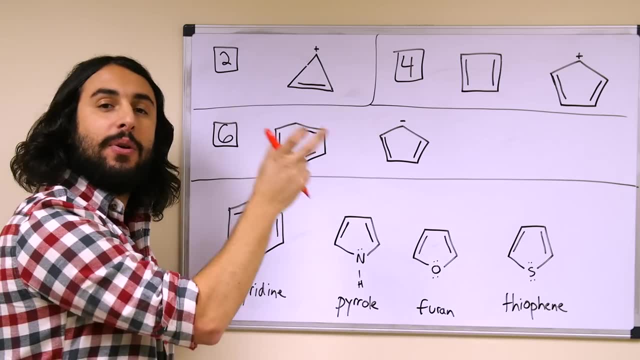 We can push that here, which would then neutralize this charge and leave the cation there, And then push the pi bond over here, Neutralizing that and leaving that there. So we could have three resonance structures of this molecule, with the cation moving amongst each carbon. 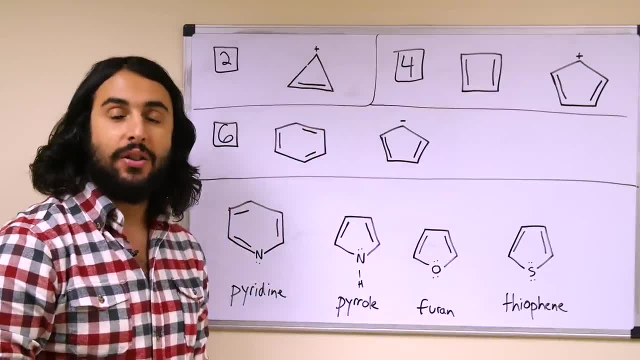 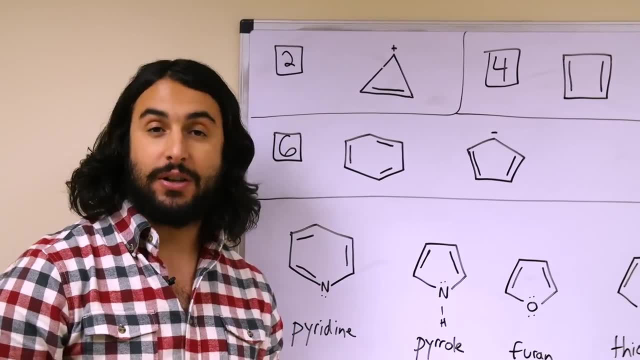 Therefore this pi bond is truly delocalized around the entire molecule. So a single pi bond here is actually fully conjugated around the molecule. So the first two criteria are satisfied, And then in addition it is only two pi electrons that are involved in resonance. 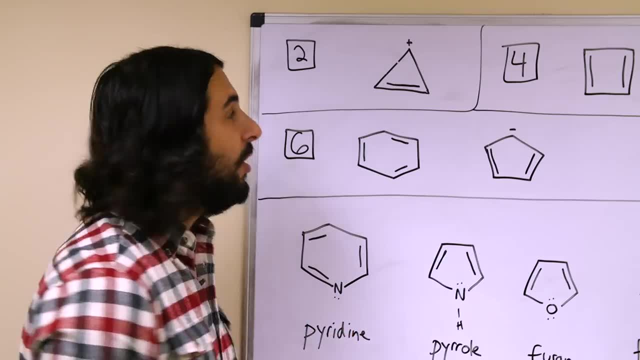 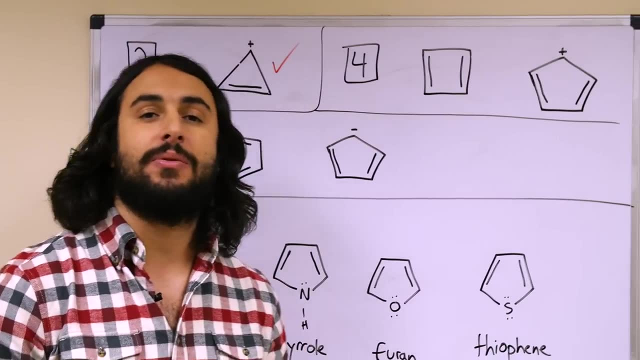 Two is a number that satisfies Huckel's rule. So this is an aromatic compound. So that works. Now, over here we look at a couple of examples involving four pi electrons that are delocalized. So over here, this is a fully planar molecule. 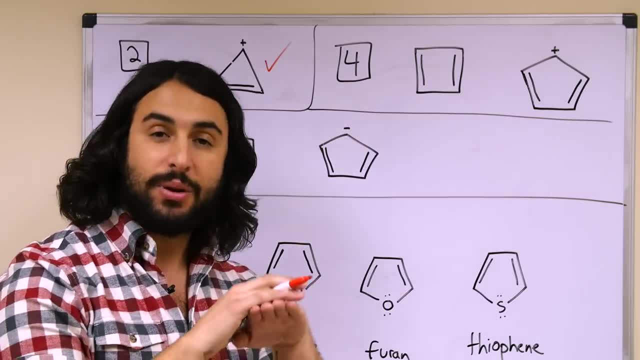 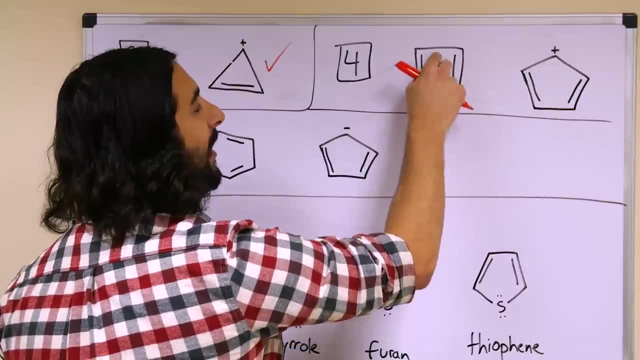 These are all sp2 hybridized carbons, So it is a completely flat molecule And it is fully conjugated. There is an additional resonance structure where we push these pi bonds to these two positions. So it is planar and fully conjugated. 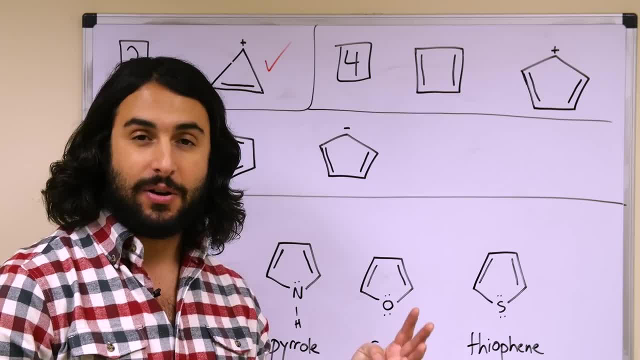 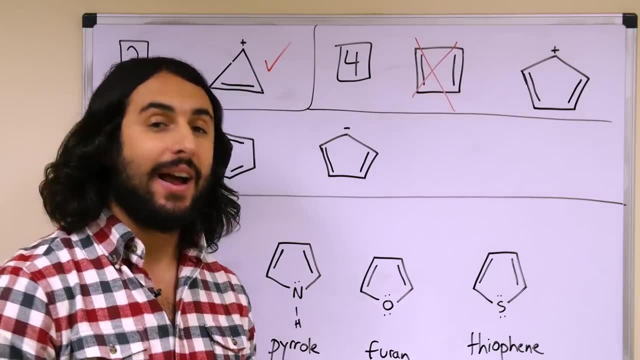 However, there are four pi electrons involved in resonance, And that does not satisfy Huckel's rule. So this is not going to be aromatic, It is going to be anti-aromatic. And then the same goes over here for this five-membered ring. 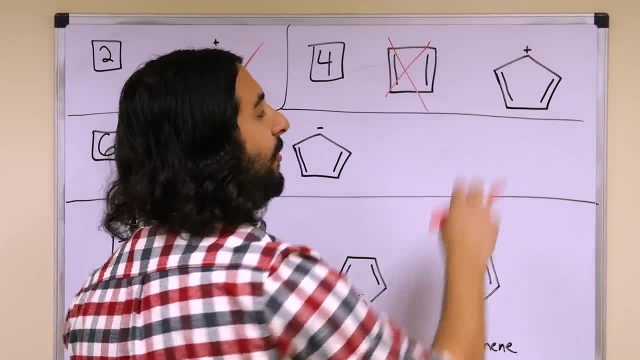 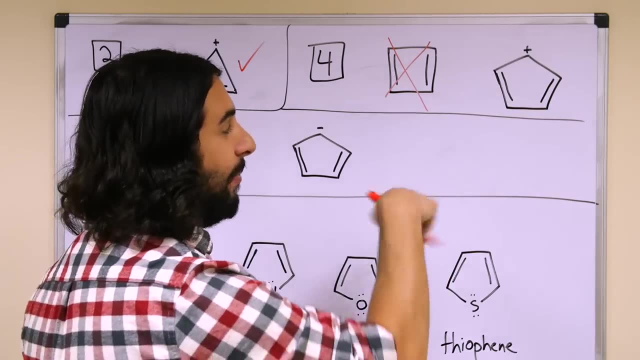 There is a cation here, So we can draw five- actually five- different resonance structures where the cation is on all of the different carbons and the pi bonds move accordingly. However, once again there are only four pi electrons involved. that does not satisfy Huckel's rule. 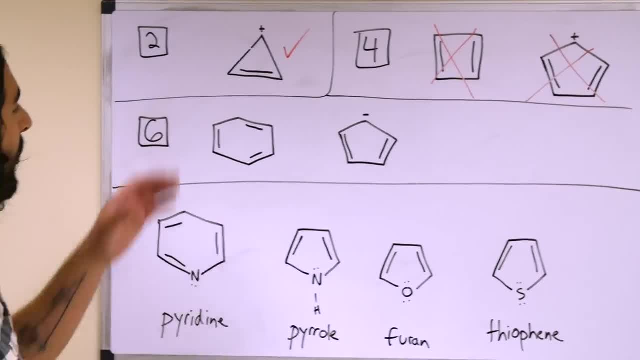 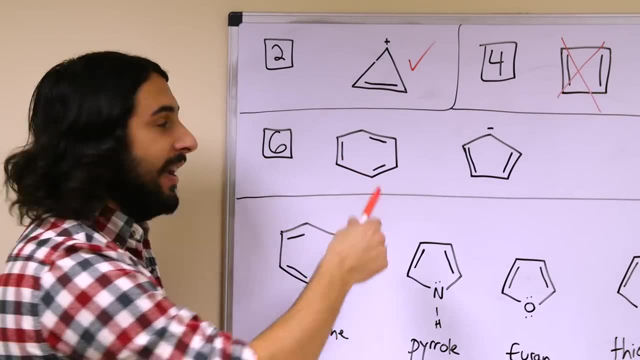 So this is not going to be aromatic. Then we look over here. We already know about benzene, But just to reiterate, we do have a situation that is fully planar. These are all sp2 hybridized carbons, So the implied hydrogens are actually in the plane of the board. 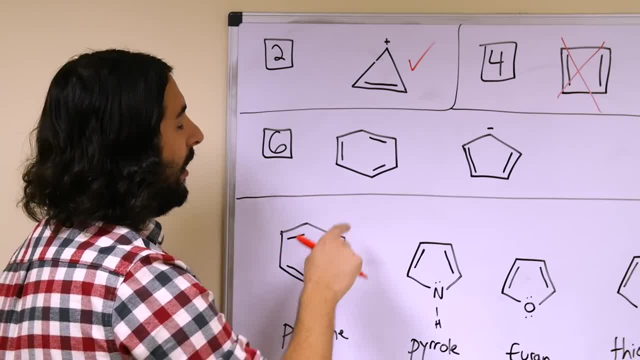 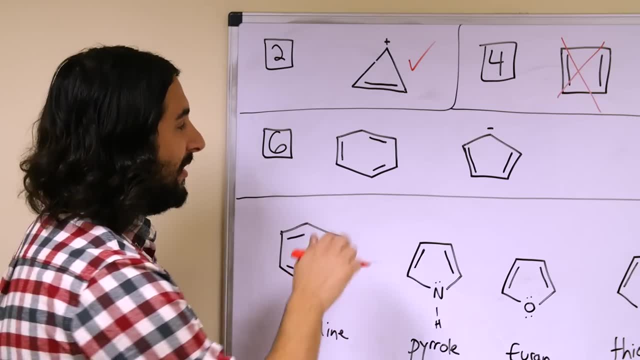 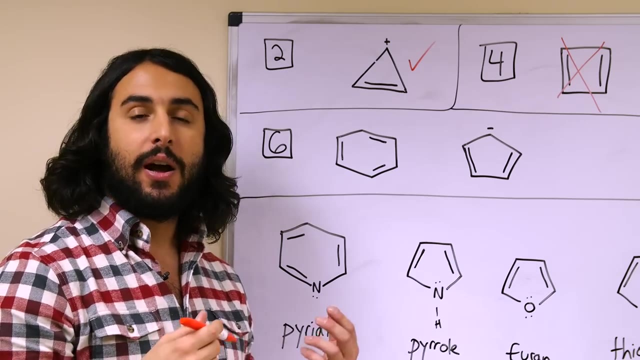 It is fully planar and it is fully conjugated. There is one more resonance structure here, where the pi bonds are in the other positions And looking at the number of pi electrons, we have two, four, six pi electrons, Remembering that every single bond, 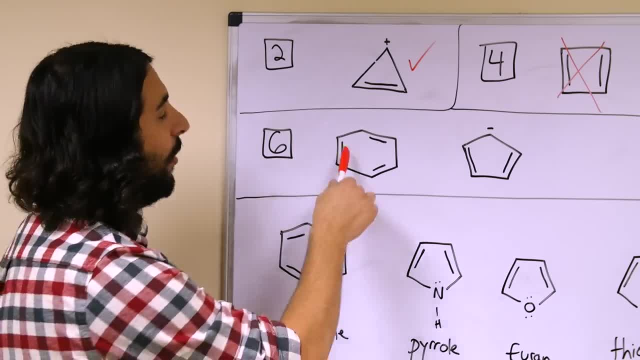 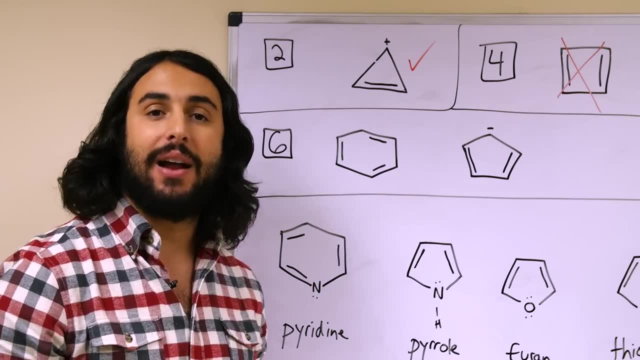 every single covalent bond has two electrons. So when we are looking at one pi bond we know that there are two pi electrons involved, So two per bond. we have three bonds, That is six pi electrons. That does satisfy Huckel's rule. 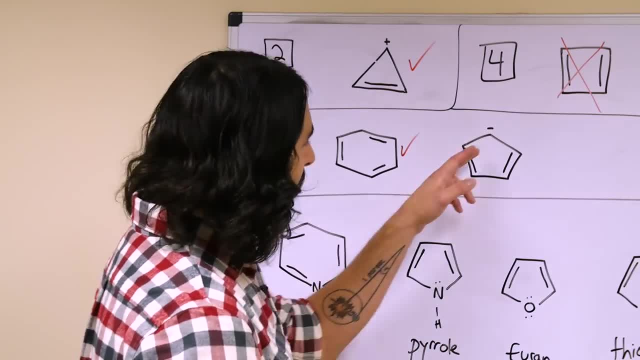 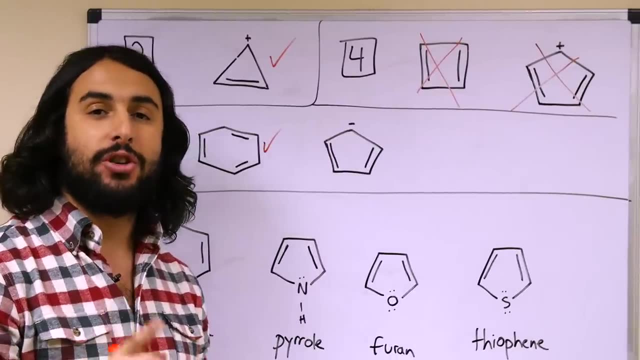 So that is going to be aromatic, as we already knew. And then over here we have the same situation as before, But now we have an anion instead of a cation, And so remember that it is not just pi bonds That can participate in resonance. 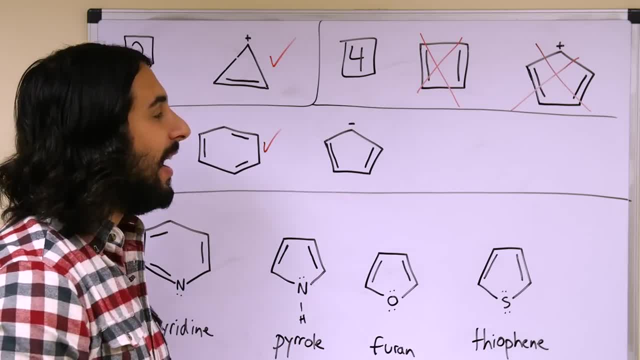 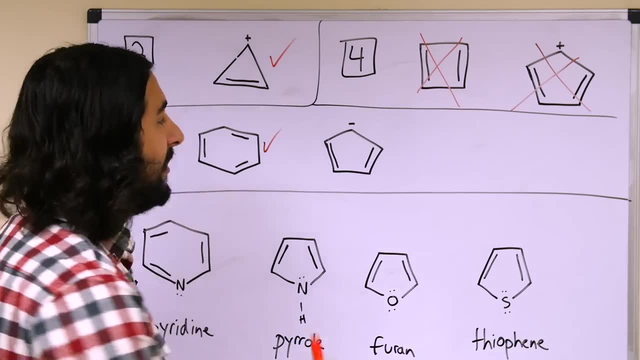 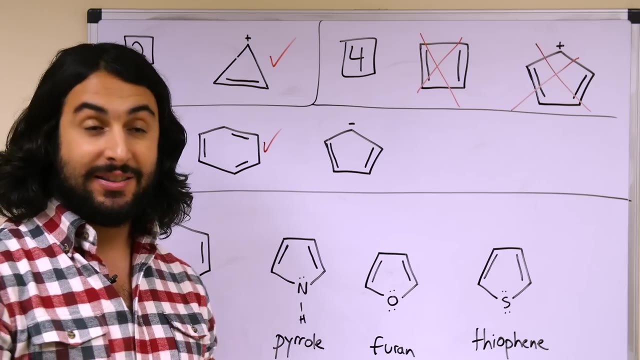 It is also lone pairs, So this negative charge implies the presence of an additional pair of electrons that are also delocalizable because they are pi electrons, And so this negative charge could go here and generate a pi bond there, Pushing this here, pushing this around, etc. 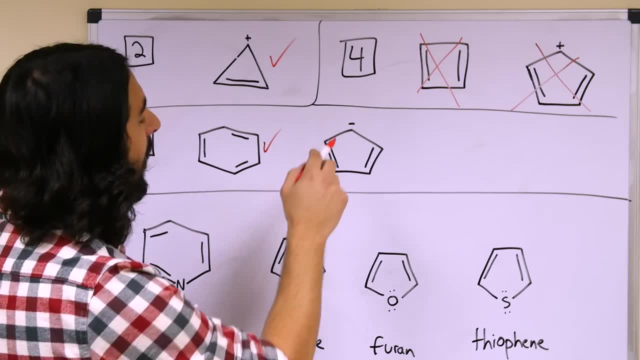 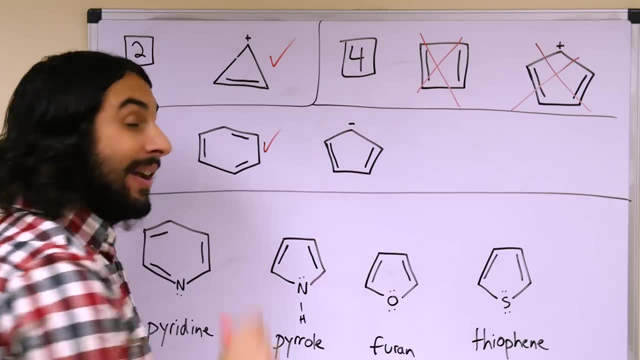 So we again could have five different resonance structures of this molecule, And so it is fully delocalizable, It is fully conjugated, And now we have two, four, six pi electrons instead of four. This is a cation, an absence of a lone pair. 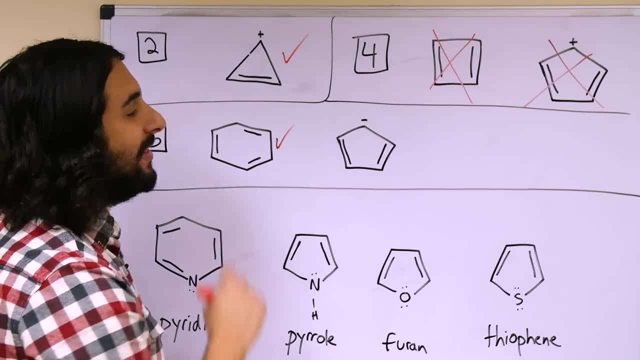 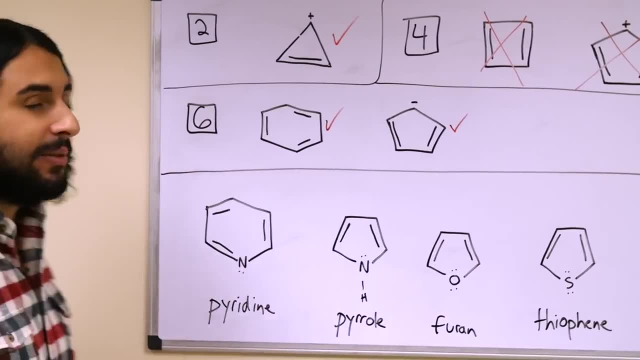 This is an anion: the presence of a lone pair. So there are six pi electrons here, And that does satisfy Huckel's rule. Now let's take a look at some of these heterocyclic compounds. So heterocyclic meaning that there are elements other than carbon. 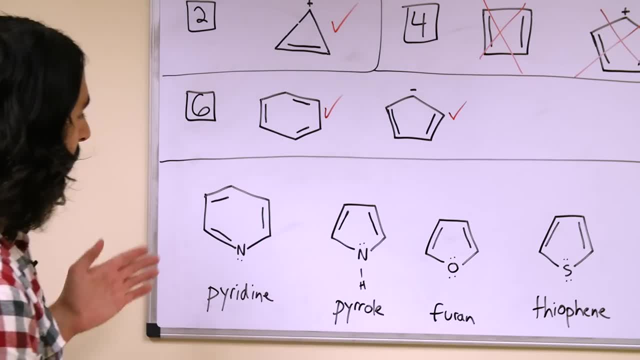 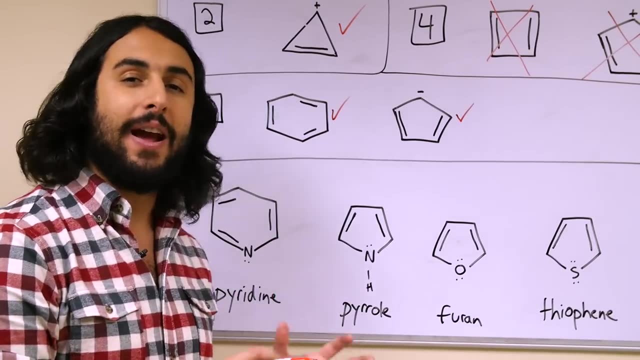 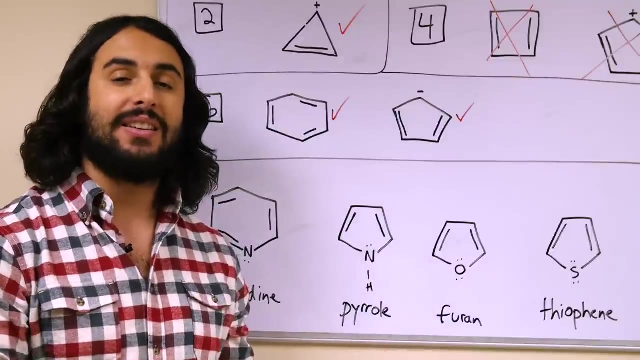 within the actual ring structure. So some of them have nitrogen, The furan has oxygen, The thiophene has sulfur, And now these can also be aromatic, because these atoms have lone pairs that may or may not be involved in resonance if they are needed to be. 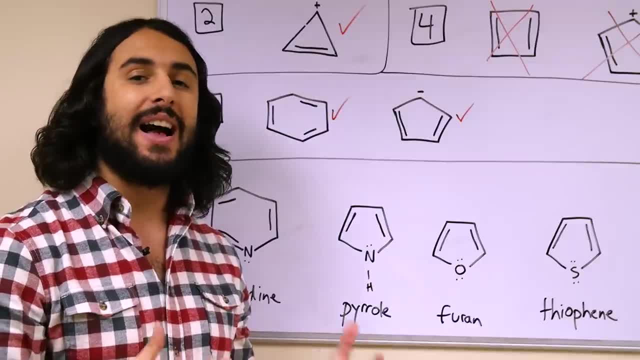 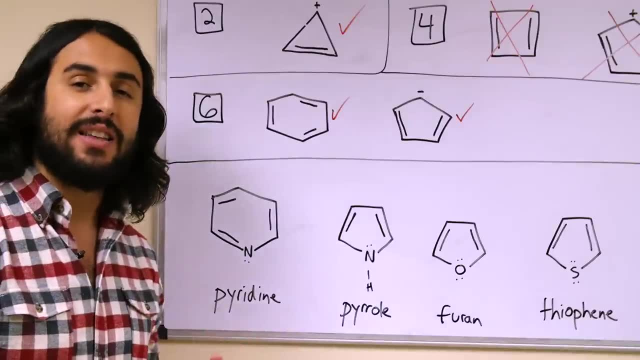 in order to generate aromaticity. Aromaticity is a highly stabilizing feature for a molecule, So if it can do it, it will. But the tricky part here is that available lone pairs need only contribute to resonance if they need to. So for example here: 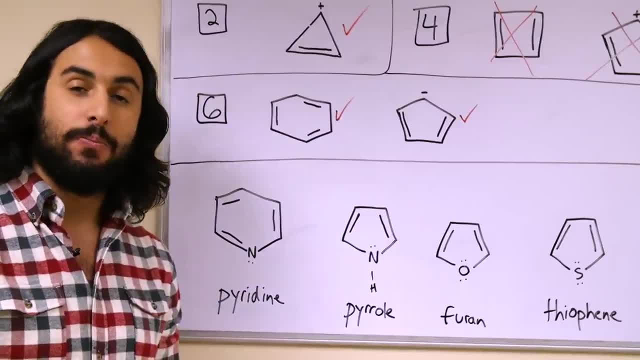 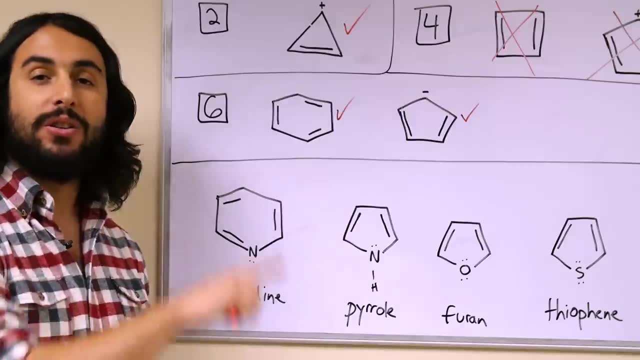 with pyridine. this lone pair doesn't need to be involved in resonance in order to generate aromaticity, So we just ignore it. These three pi bonds are going to be able to delocalize and generate aromaticity on their own. However, in this situation, 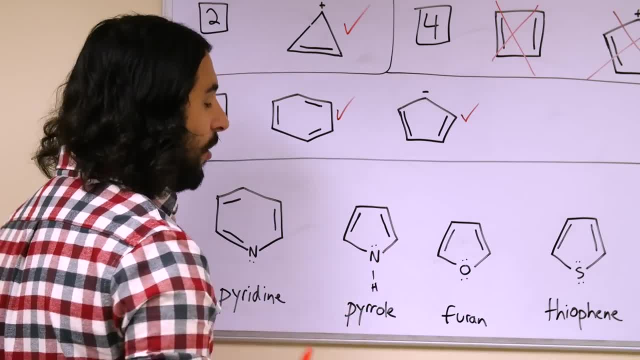 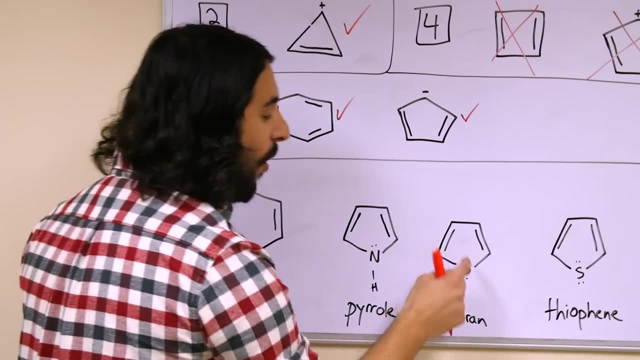 and actually all of these situations, one lone pair, the only one available here for this nitrogen atom will be needed and able to generate aromaticity Over here. one of the two, and in this case as well, one of the two lone pairs.